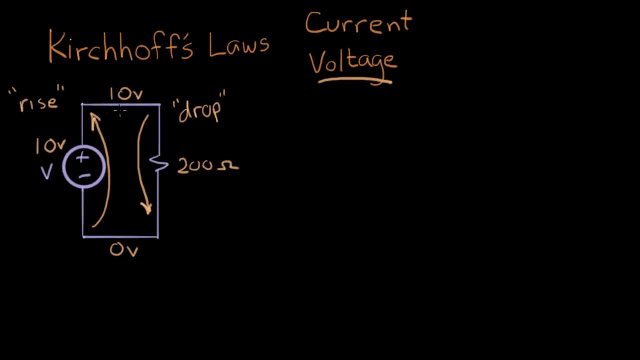 If I look at this voltage rise- here it's 10 volts. and if I look at that voltage drop, the drop is 10 volts. I could say the drop is 10 volts. or I could say the rise on this side is minus 10 volts. 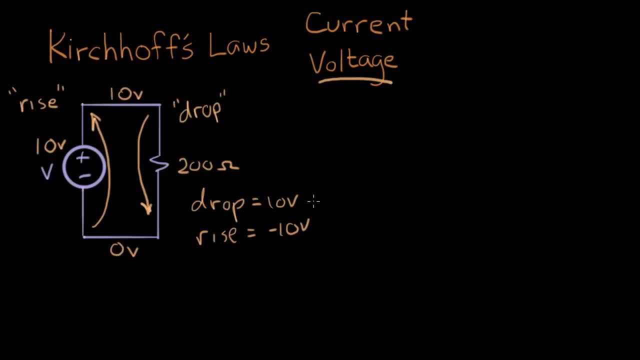 A rise of minus 10.. These two expressions mean exactly the same thing. It meant that the voltage went from 10 volts to zero volts, sort of going through this 200-ohm resistor. So I write a little expression for this. 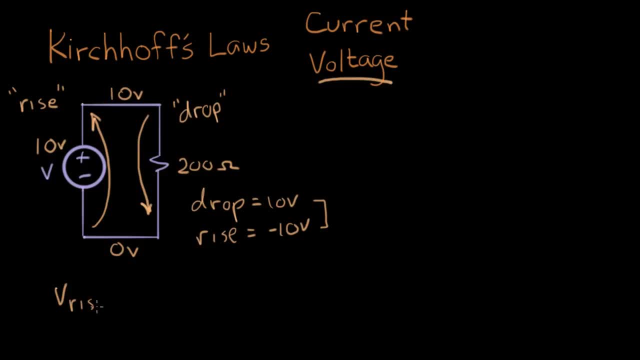 which is vrise minus vdrop, equals what Equals zero. I went up 10 volts, back down 10 volts, I end up back at zero volts, and that's this right here, And this is a form of Kirchhoff's voltage law. 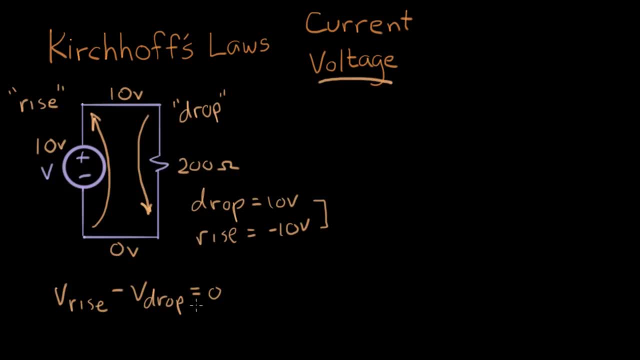 It says the voltage rises minus the voltage drops is equal to zero. So if we just plug our actual numbers in here, what we get is 10 minus 10 equals zero. I'm gonna draw this circuit again. Let's draw another version of this circuit. 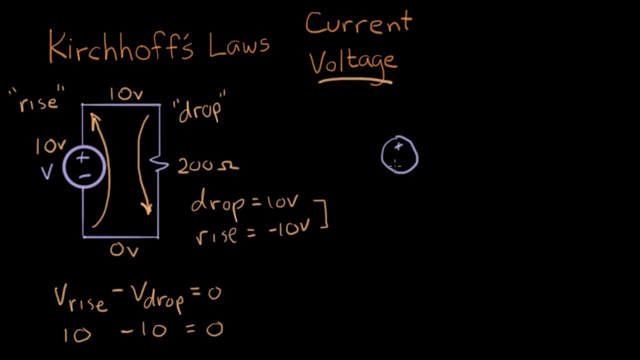 and this time we'll have two resistors instead of one And we'll make it whoops. We'll make it two 100-ohm resistors And let's go through and label these. This is again 10 volts. 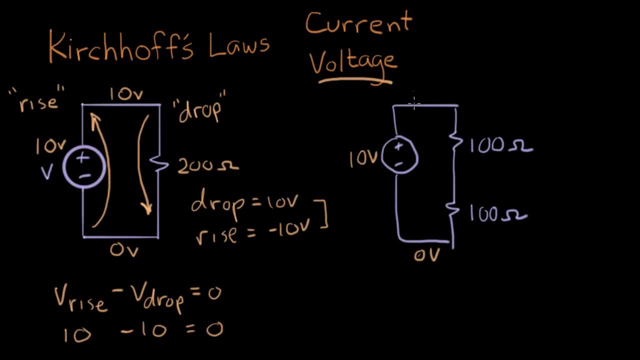 So this node is at zero volts. This node is at 10 volts. What's this node? This node here is: these are equal resistors, so this is gonna be at five volts. That's this, This node. voltage here with respect to here. 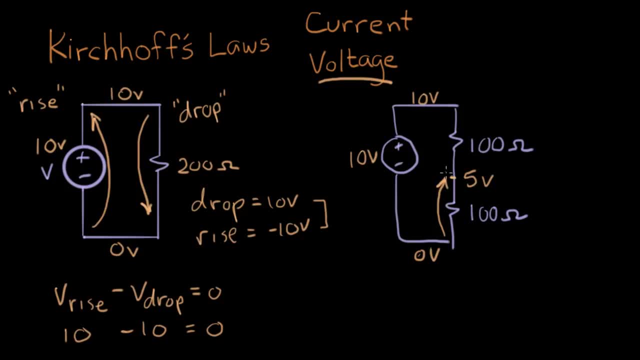 So that is five volts, This is five volts And this is 10 volts. So let's just do our visit again. Let's start here and count the rises and drops. Okay, we go up 10 volts, Then we have a voltage drop of five. 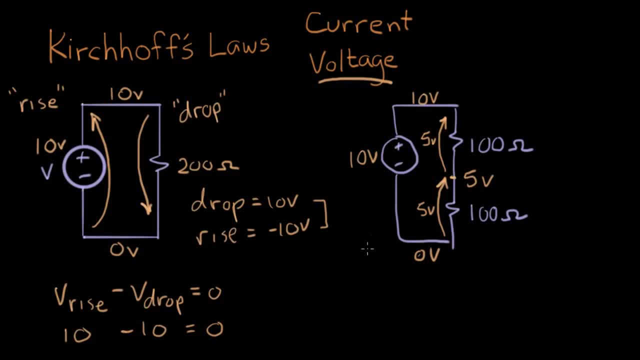 And we have another voltage drop of five And then we get back to zero. We can write the sum of the rises and the falls, just like we did before. We can say: 10 volts minus five. minus five equals zero, All right. 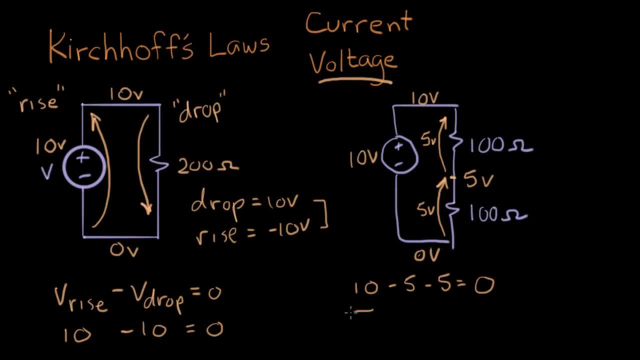 So I can generalize this. We can say this in general. We can do: the summation, That's the summation symbol of the V rise minus the sum of the V fall equals zero. This is a form of Kirchhoff's Voltage Law. 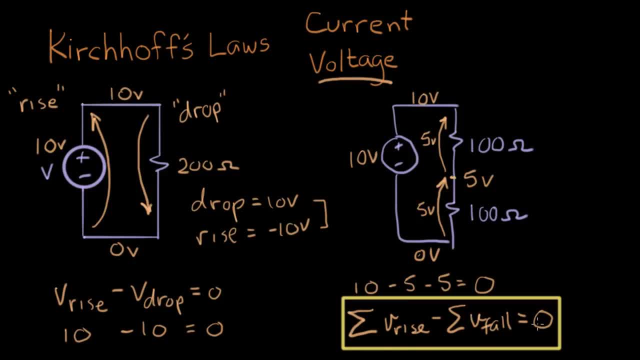 The sum of the voltage rises minus the sum of the voltage falls is always equal to zero. There's a more compact way to write this that I like better, And that is: we start at this corner. We start at any corner of the circuit. 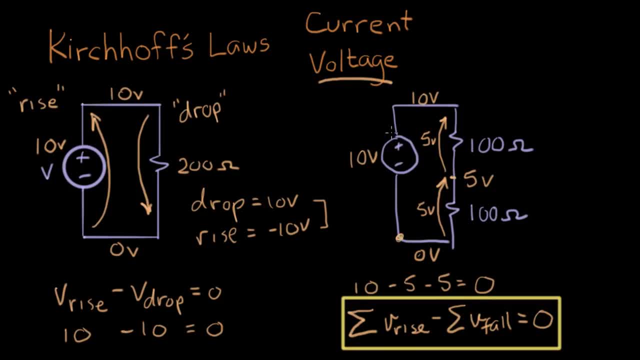 Let's say we start here. We're gonna go up 10 volts, down five volts and down five volts. So what we're adding is the voltage rises. We're adding all the voltage rises Rise plus 10. That's a rise of minus five and a rise of minus five. 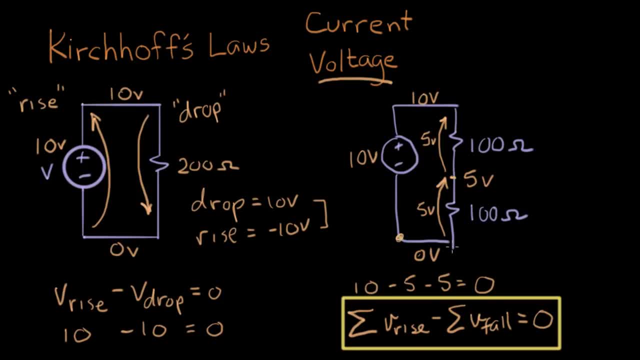 So I can write this with just one summation symbol. The voltage is around the loop, So I can write this with just one summation symbol: Where I takes us all the way around, the loop equals zero. So this means I start any place on the circuit. 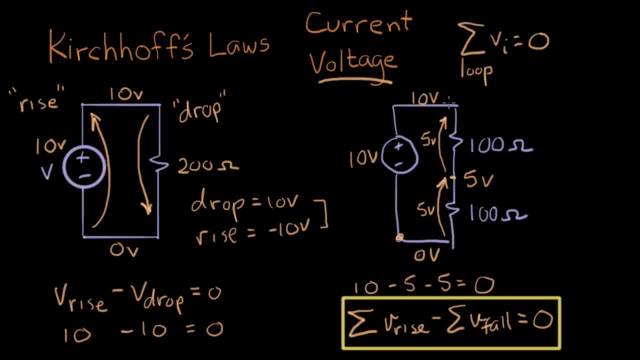 go around in some direction this way or this way- up, down, down, and I end up back at the same voltage I started at. So let's put a box around that too. This is KVL Kirchhoff's Voltage Law. 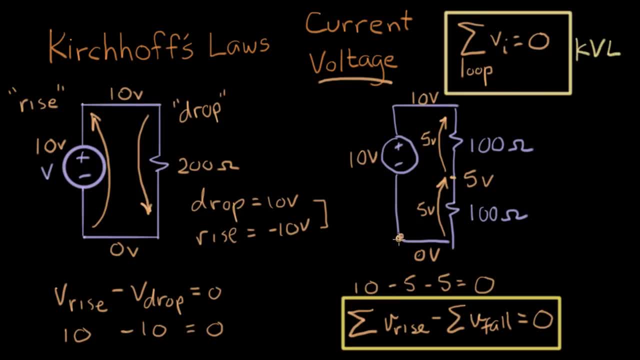 Kirchhoff's Voltage Law. Now I started over here in this corner, but I could start anywhere If I started at the top and went around clockwise. if I started here, say, I would go minus five, minus five plus 10,.